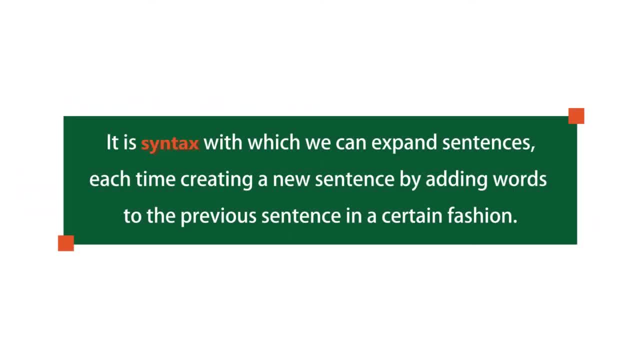 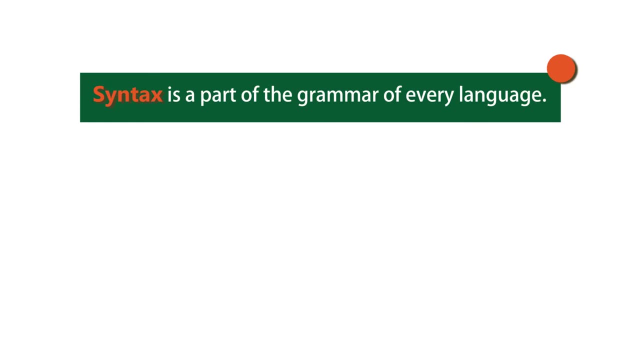 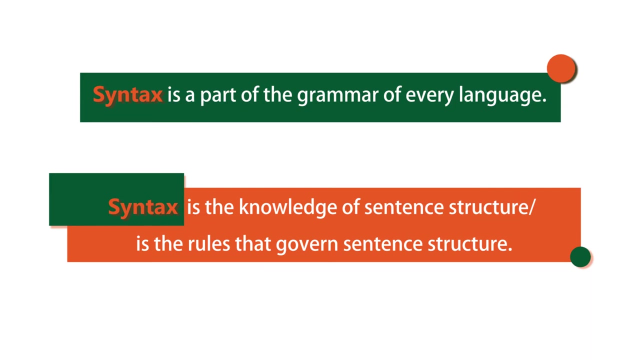 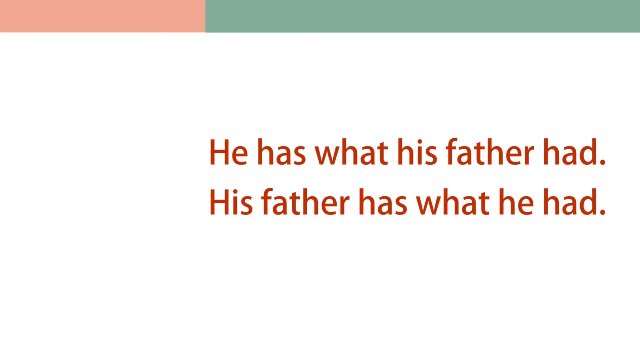 But my point here is that, in a way, it is our knowledge of syntax that we are applying for creating increasingly more complex sentences. Syntax is part of the grammar of every language And it consists of the speaker's knowledge of sentences and their structure. He has what his father had. His father has what he had. Because of syntax, it is possible to have. 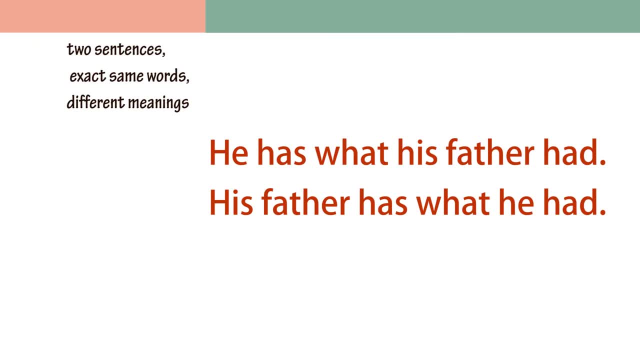 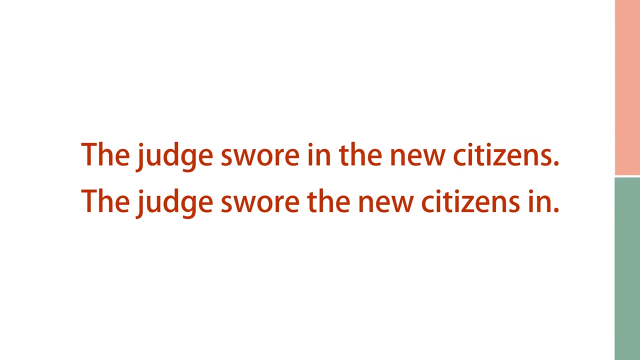 two sentences with the exact same words but two different meanings. In this case, if you want to get more imaginative, you can think of syntax as a dimension, as an extra dimension that sits on top of these words and constructs a particular relationship between the words. Sometimes you may actually have two sentences with two different orders that mean the exact. 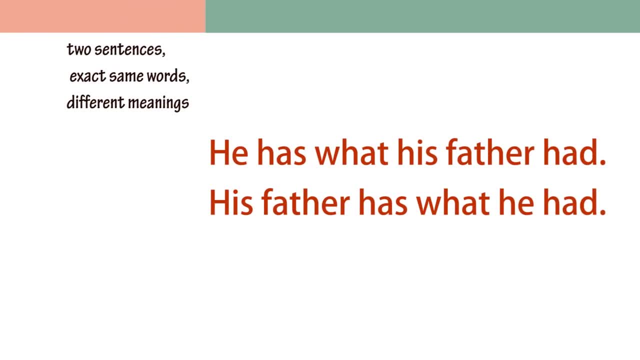 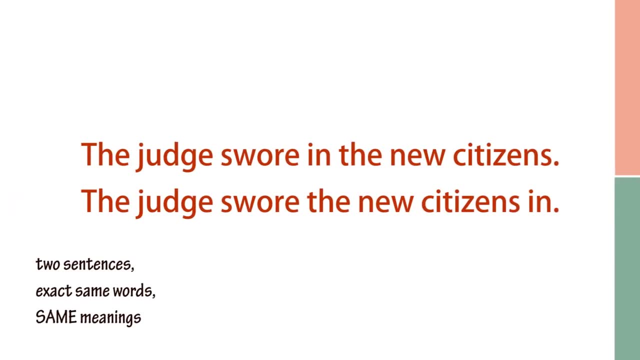 same thing. You see, in the you had two sentences with the same words, different orders, meaning two different things. But here you have two sentences with this exact same words and different orders, but they still mean the same thing. So here syntax allows us to have the same interpretation of. 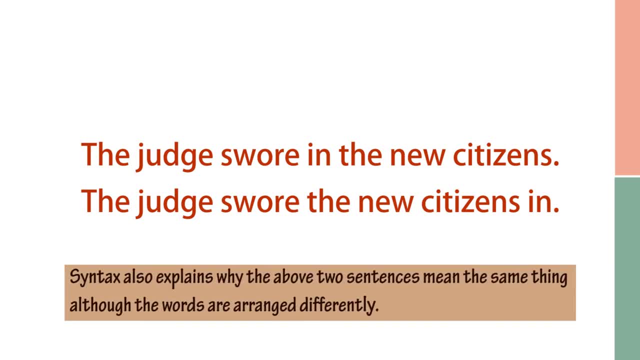 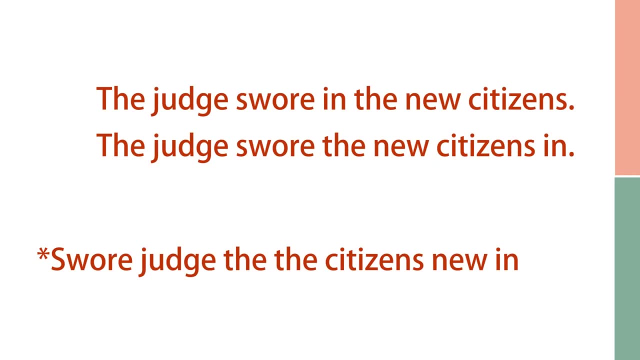 two different word orders. It is also the syntax that tells us that here in this sentence, although we have the same words that we had in the above two sentences, the arrangement of words we have here is not acceptable in English. If you say swore, judge the, the citizens knew in, this is not acceptable in. 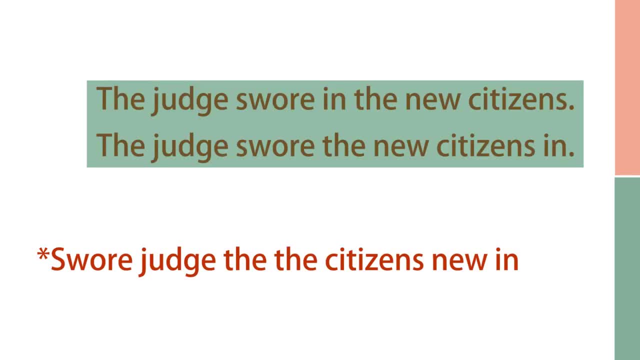 English. So although the two differing word orders above were acceptable- both were both acceptable and rendered the same meaning- it doesn't mean that any random order of words is acceptable. That is also what is the realm of syntax. So keep in mind that we are having an interface or we are interacting with. 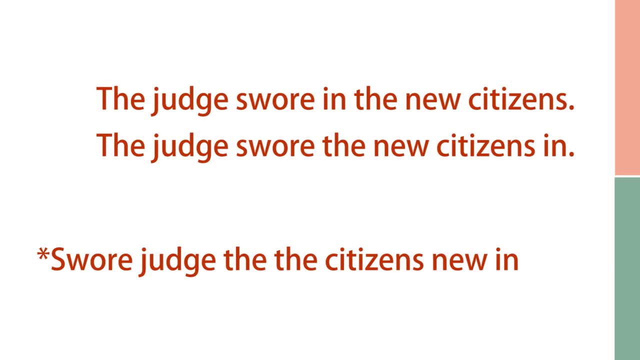 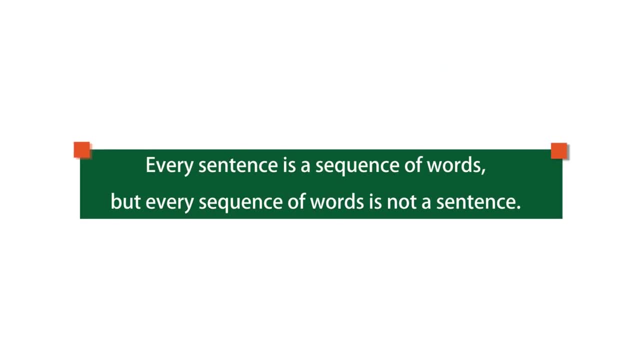 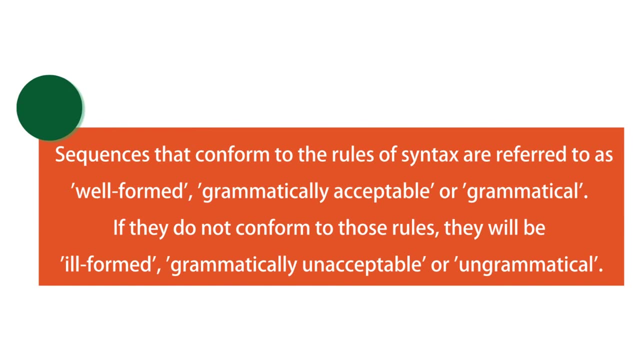 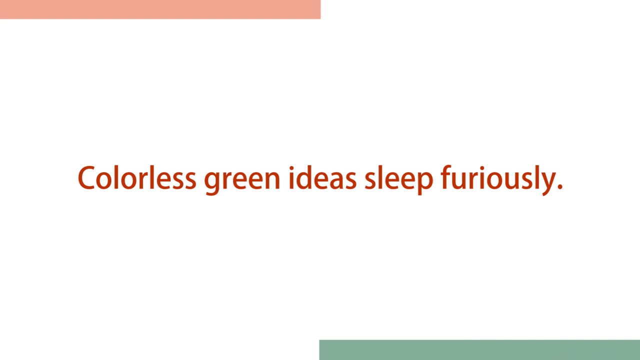 the semantics. but syntax is not about the meaning. The discussion of meaning is a semantics which we will cover in the future. So every sentence is a sequence of words, but every sequence of words is not a sentence. Sometimes a sentence may be grammatical but may not be meaningful. Why it is nonsensical will be explained. 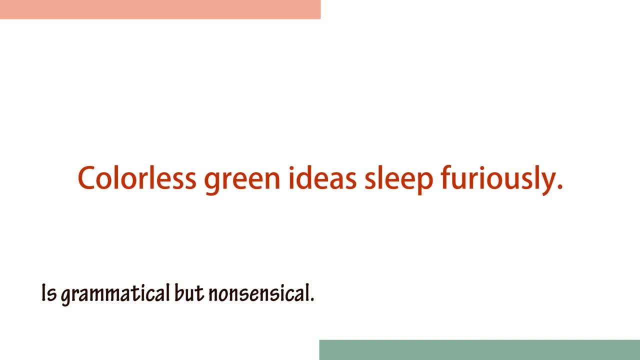 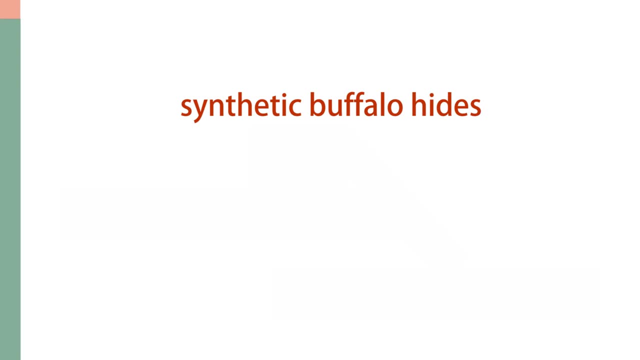 there are in the realm of semantics, but this sentence is grammatically well formed. Also, if I tell you synthetic Buffalo hides, what does synthetic Buffalo hides mean? So syntax here tells us that synthetic Buffalo hides its ambiguous and has the following two possible meanings. It mean, it could mean, synthetic hides. 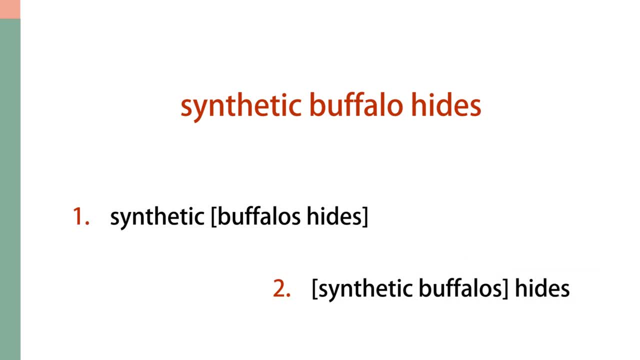 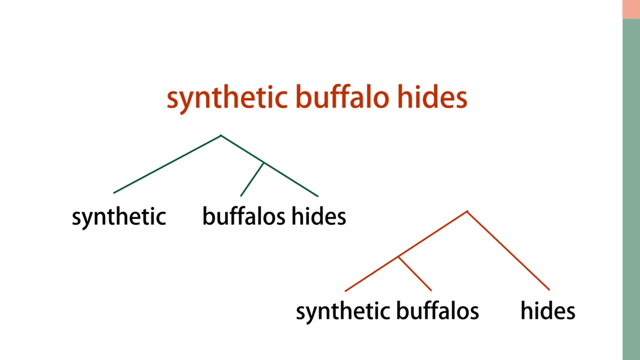 of Buffaloes, or it could mean hides of synthetic Buffaloes. The same syntactic knowledge can be represented using diagrams, the tree diagrams. So these syntax trees of sentence or phrases structure, in this case phrases structure, are similar to morphology trees for word structures. 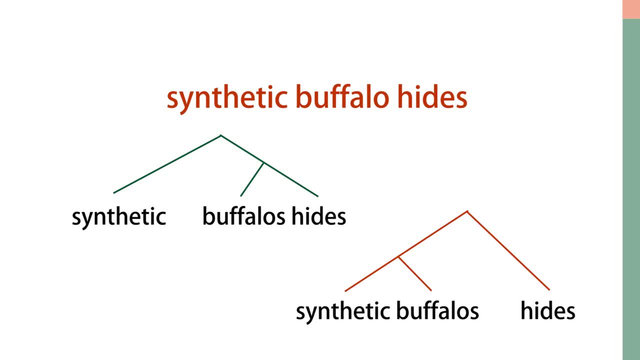 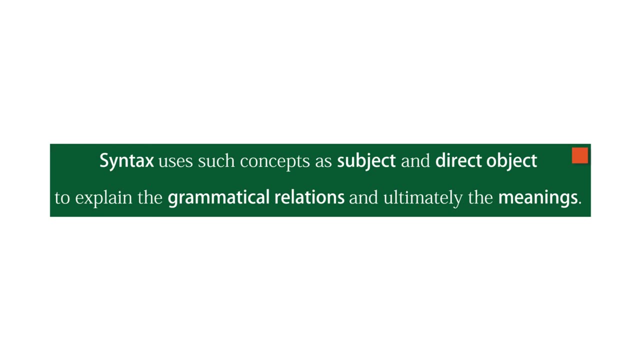 But here The tree structure, the syntax tree. this tree diagram explains the phrase structure, It could explain the sentence structure And I can wrap up the discussion by letting you know that syntax uses such concepts as subject and direct object to explain the grammatical relations and ultimately the meanings of John killed Mary as opposed to Mary killed John. 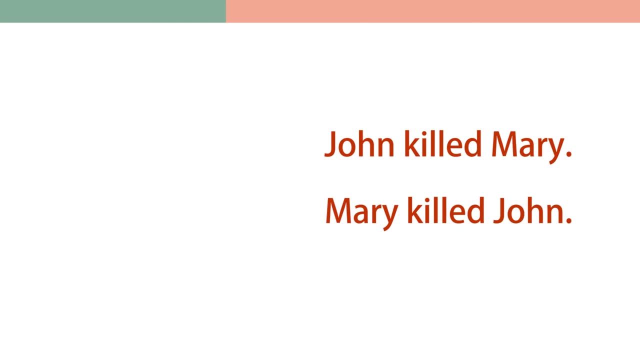 So in this context, Syntax can have serious legal consequences, Because you want to know who killed who. In one, John is subject and in two, Mary, and the direct objects are Mary and John respectively. In a sense, if you want to find out who the killer was, you need to find out what the subject is.